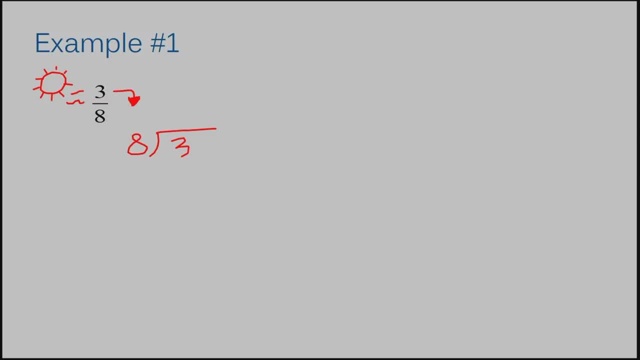 The top number always goes inside, So the top number always gets blown over to the right. Now it's time to divide. Eight can't go into three, So you have to add a decimal zero. I always bring my decimal up. 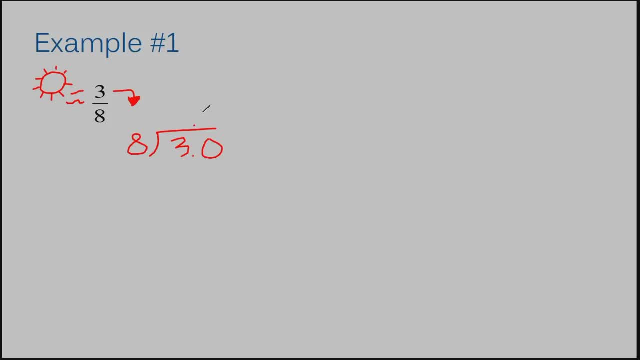 Now, eight can go into thirty. It goes into it three times And that's twenty-four. When you subtract you get six. Add another zero to bring it down. Eight goes into sixty seven times And that answer is fifty-six. 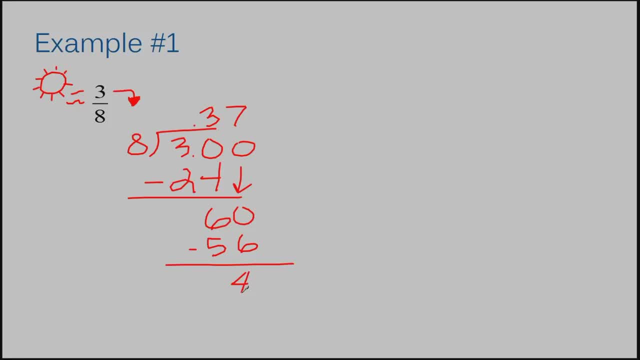 When I subtract I get four. Add another zero, Bring it down. I'm going to extend my line up here. Eight goes into forty five times, So the decimal form of three-eighths is three hundred seventy-five thousandths. 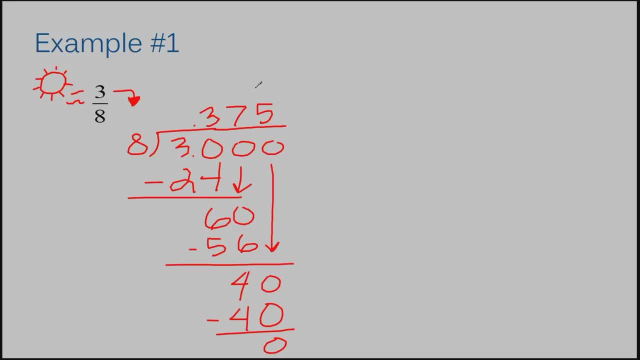 Now I also need the percent form of this number. So at this point we have two options. We can either take our fraction to a percent or our decimal to a percent. I think it's easier to take the decimal to a percent. 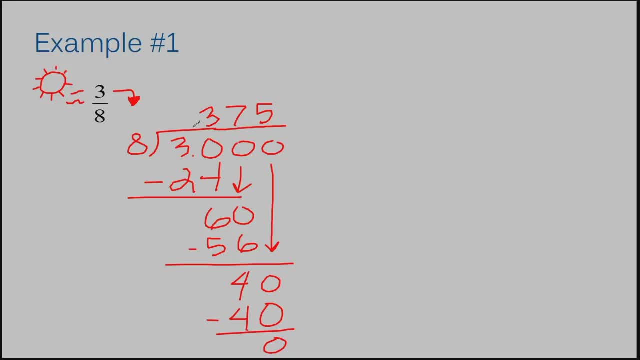 To go from a decimal to a percent, all you do is move your decimal space over two spaces to the right. So we start with something that looks like this: Three hundred seventy-five thousandths Equals thirty-seven and five-tenths percent. 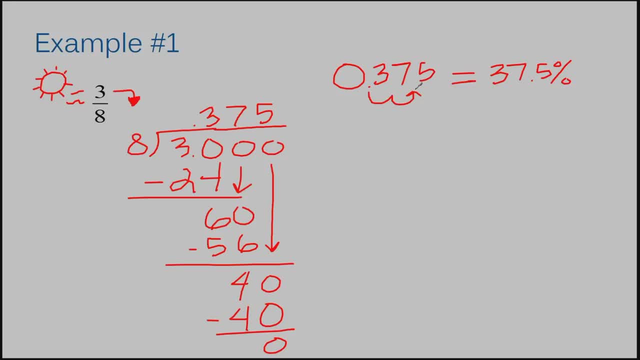 So all I did was move my decimal over two spaces and added my percent sign. So if I needed to use these numbers interchangeably- Let's say I had a problem where a decimal was more useful- I could take my fraction and turn it into a decimal. 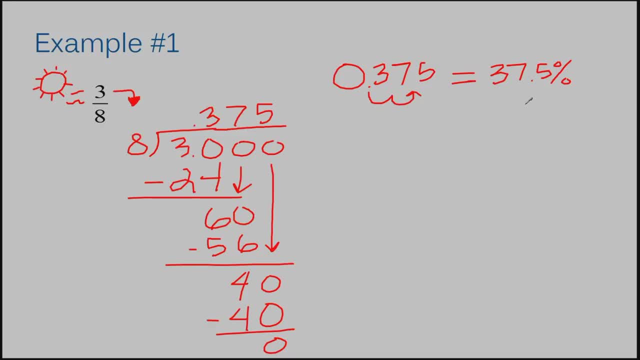 Or I have a problem where having my number as a percent would be more useful. I could change my fraction into a percent. It may be a two-step process. You may have to take that fraction into a decimal and then to a percent. 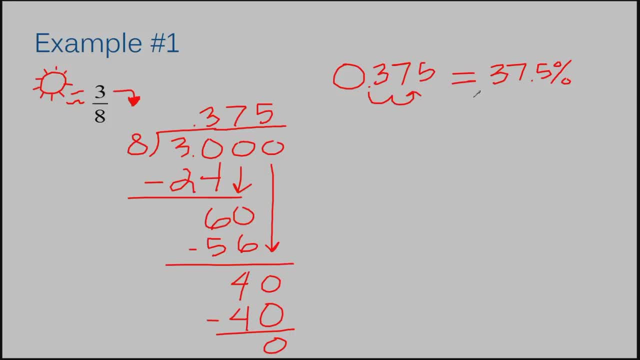 And that's fine. Really, you're just doing what you need to to put everything in a form that is best for you. So the number is three-eighths, Three hundred seventy-five thousandths And thirty-seven and five-tenths percent are all equal to each other. 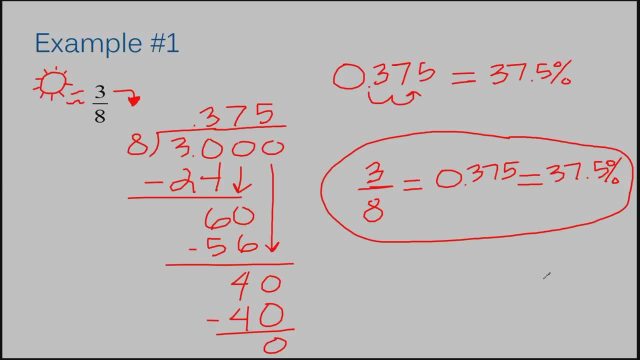 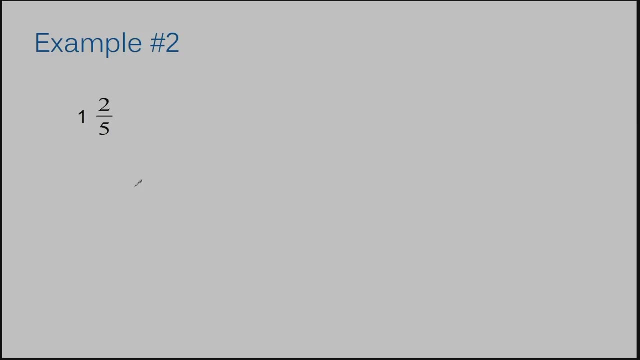 So anytime you're given a problem, You are free to convert the number to any form that you need to To make it easier for you to work with. Let's move on to example number two. Example number two: I have one and two-fifths. 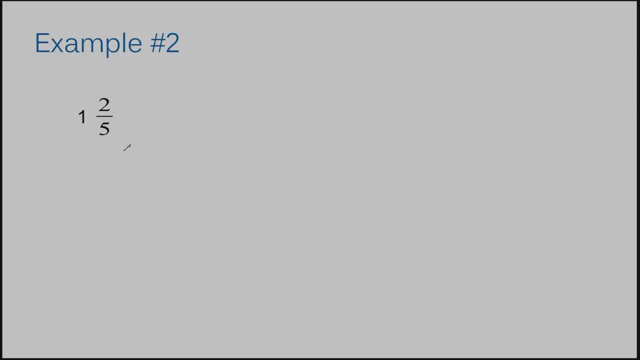 I'm going to convert that to a decimal. To begin with I have a whole number of one, So that whole number is just going to come out in the beginning. I only need to convert the fraction portion to a decimal, And then the whole number will just be added to the fraction portion. 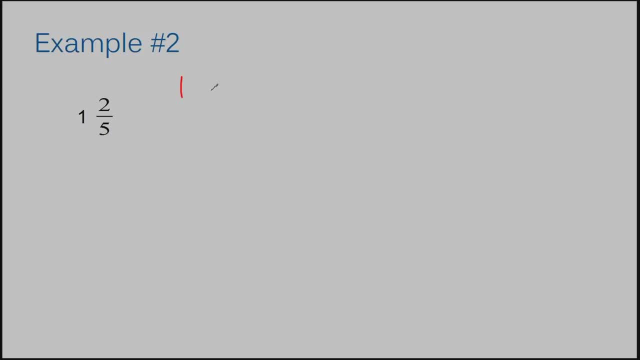 So it will be one, And then there will be a decimal, And then whatever I got as the decimal version of this- Remember, if it's sunny and windy on my left, The top number gets blown over to the right. 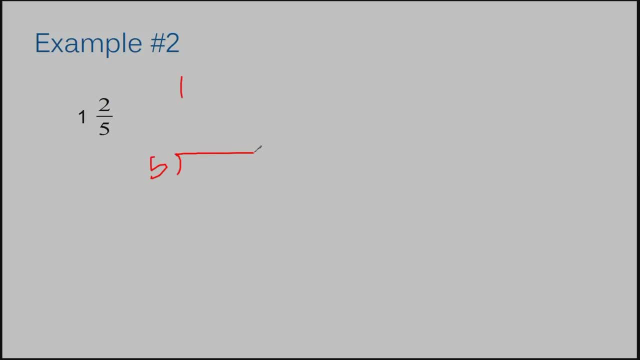 So I have five And it goes into two. Five cannot go into two, So I have to add a decimal zero. Bring my decimal up: Five goes into twenty Four times And it is twenty. I subtract. 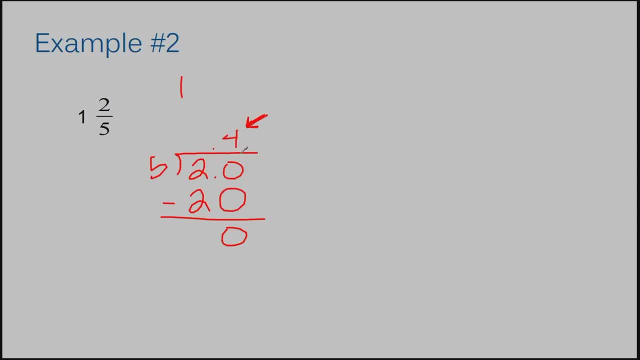 And I get zero. So I'm done. So the four-tenths is the decimal form of my two-fifths, So I'm going to add that to the whole number of one. So as of now, 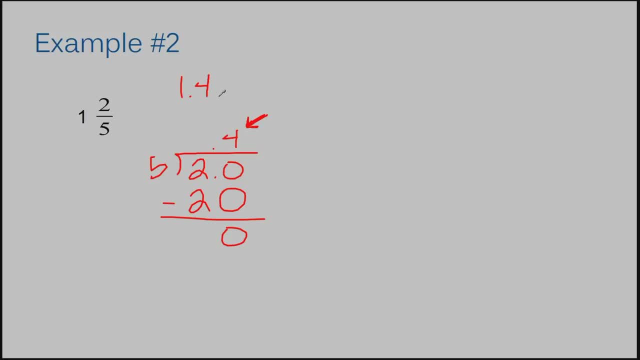 I have my fraction form of the number And I have my decimal form of the number. Now I need to get my percent form of the number. I'm going to start by writing my number And I'm starting with the decimal form of it. 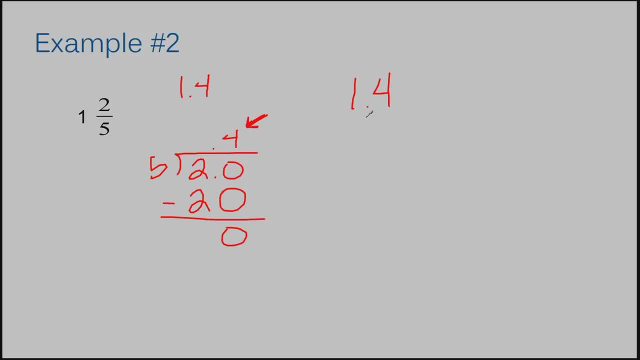 I'm going to move my decimal over two spaces to the right. I have to add a zero, because there's an extra space here, And I end with one hundred forty percent. So my three forms of this number are one and two-fifths. 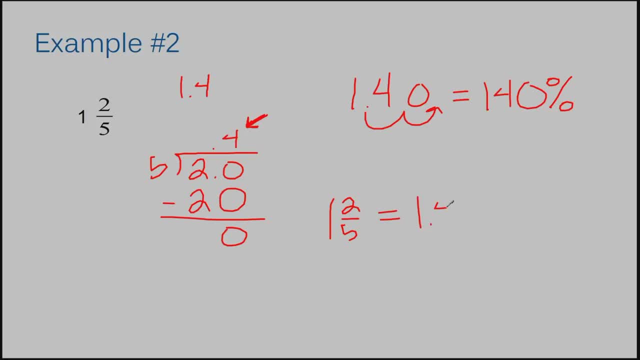 Which is equal to one and four-tenths, And that's equal to one hundred forty percent. Let's move on to example number three. For example number three, we start with an improper fraction. That's no problem, We can still use all of the same steps. 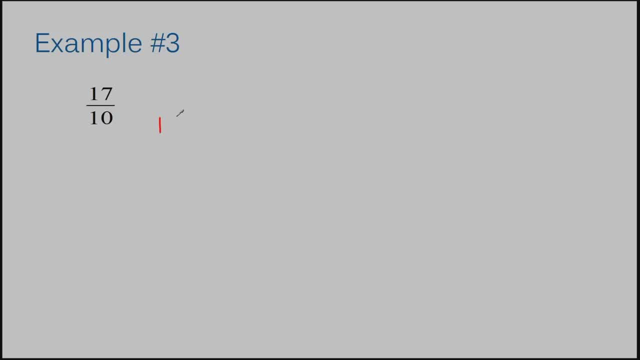 Remember it's sunny and windy. The top number gets blown over, So we have a ten And it goes into our seventeen. Ten can go into seventeen, So I don't need to add a decimal zero. It goes in one time. 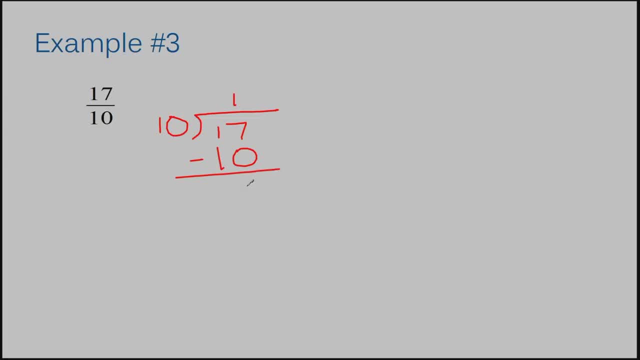 And it's ten. When I subtract, I get seven. Now, because I've subtracted And I didn't end up with a zero, I know that I need to add a decimal zero, So I have something to bring down. 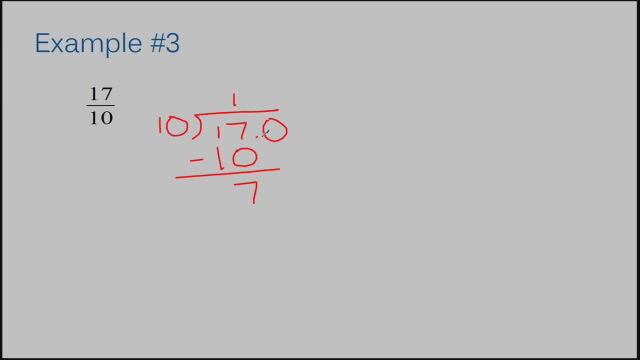 As soon as I write my decimal zero, I like to bring my decimal up immediately, So I don't forget to add it later. Now I can bring down my zero. Ten goes into seventy Seven times And it is seventy. 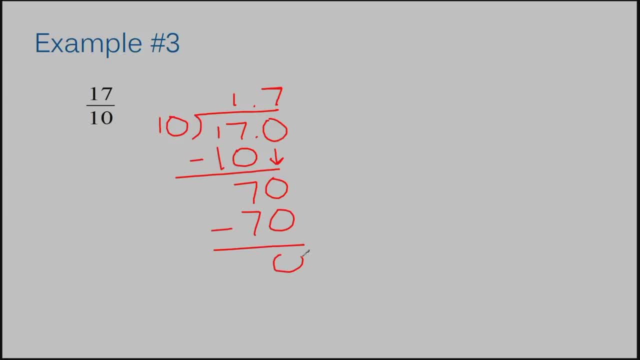 When I subtract, I get zero. That's a good sign that I solved correctly. If I end with a zero And there's nothing else to bring down, That's a good sign that I probably solved my answer correctly. So right now we have our fraction form of the number. 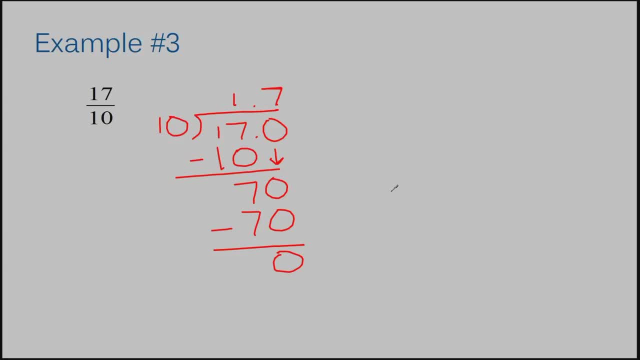 Our decimal form. And now we need to get our percent form. Remember to get our percent form. All we do is move our decimal space over two places to the right. So I write my number down: One and seven tenths. 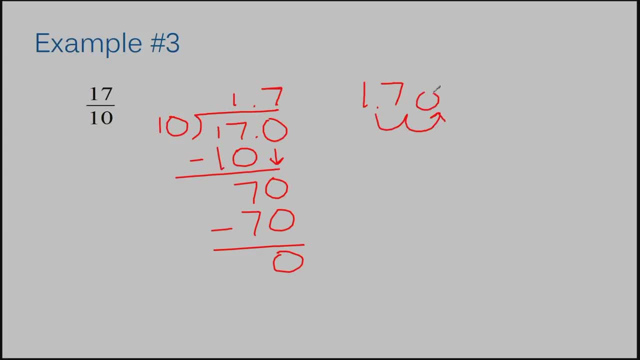 And now let's move our decimal over two spaces to the right. Add a zero, Because there's an empty space there, And that equals One hundred seventy percent. So I have seventeen tenths. That equals One. 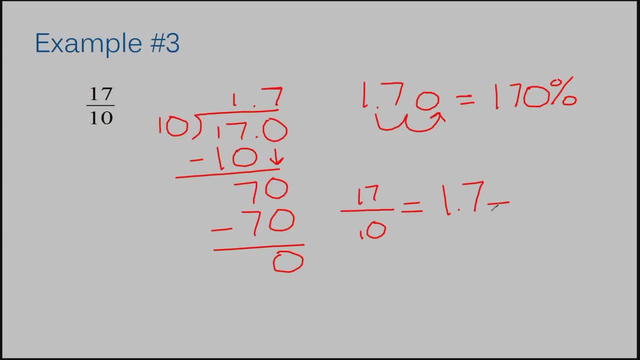 And seven tenths, Which also equals One hundred seventy percent. And I do want to point out something: Please don't think that the seventeen tenths is only equal to the one and seven tenths, Because they're touching each other. 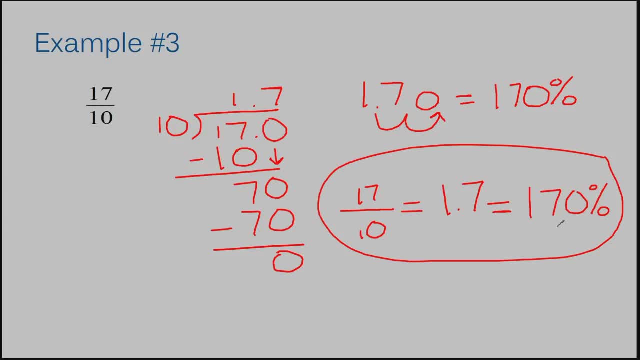 The seventeen tenths also equals the one hundred seventy percent. All three of these are equal in value. It doesn't matter really where they're positioned. This is sort of like saying: This is one dollar, This is four quarters And this is ten dimes. 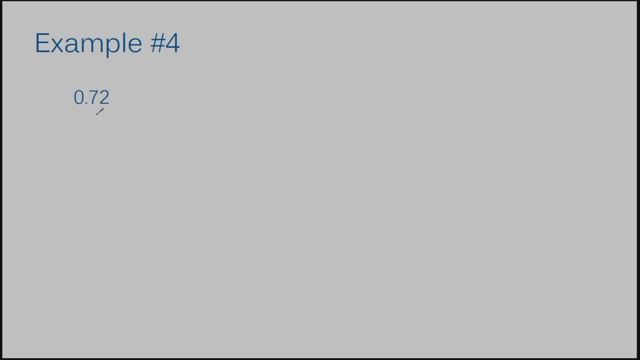 Let's move on to example number four. I have seventy two hundredths, So this time we're starting with a decimal. Is that a problem? Definitely not. All I need to do is move my decimal over two spaces to the right. 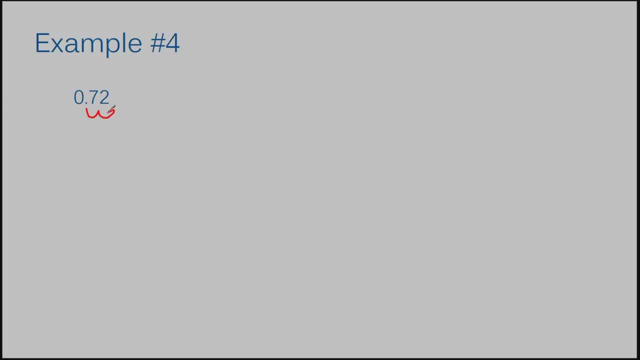 To get a percent One, two, So that equals seventy two percent. How do I get a fraction out of this? Remember, when you say the name of a decimal in the correct way, You always say the name of the place of the very last digit. 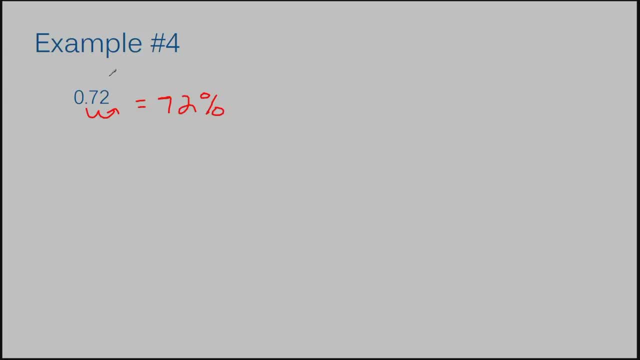 So this is seventy two hundredths, Meaning the two is in the hundredths place. So one hundred is the denominator that I would give this number. So you write the number down without the decimal And you give it. You give it a denominator of one hundred. 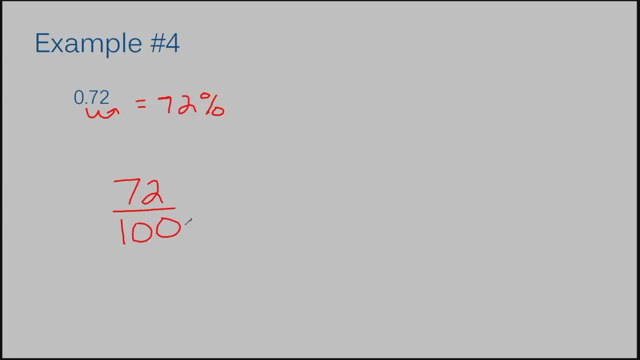 This is the fraction form. The only problem with this fraction is it's not simplified. So I'm going to simplify. To simplify, I'm going to divide the numerator and the denominator by two, And after doing that, I get thirty six over fifty. 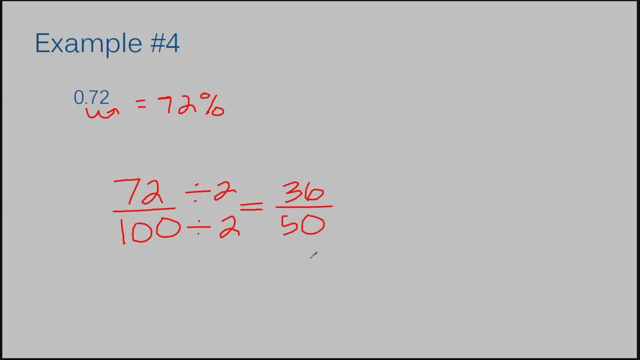 Thirty, six and fifty are both even numbers, So that means I can simplify this fraction again. If I had originally divided by the greatest common factor to simplify here, Then I would have only had to simplify one time. But because there was a number that was larger than two, 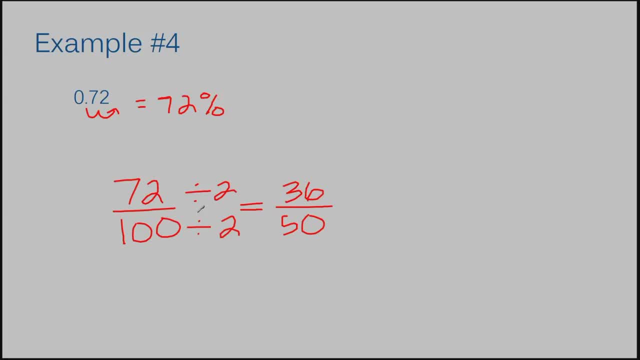 That could have gone into the seventy two and the one hundred. It makes me have to simplify more than one time. So, because they're even, I'm going to divide by two again And I get eighteen over twenty five. This cannot be simplified anymore. 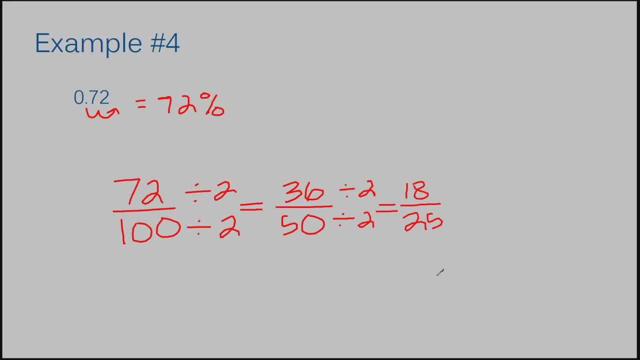 There's no number that goes into both eighteen and twenty five, So the three forms of my number are Seventy two hundredths, Seventy two percent And eighteen over twenty five. Let's move on to example number five. I have eight and one tenth. 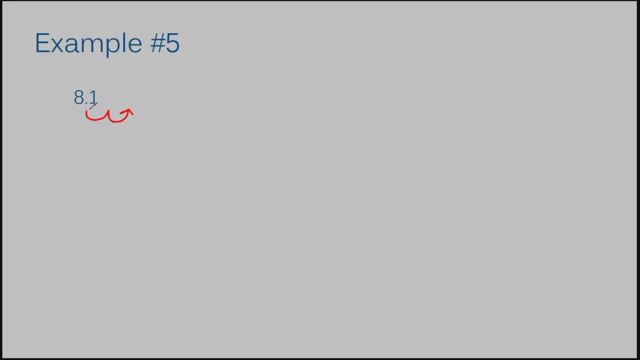 I'm going to change this into a percent. first I move my decimal over two spaces to the right, Add a zero And a percent sign. That looks like eight hundred ten percent. I need to make this into a fraction, Remember. 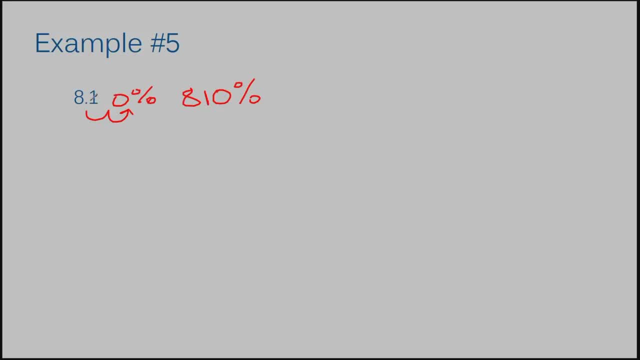 The way you say your decimal. Your decimal gives you a hint At what your fraction is going to look like. I'll go ahead and tell you something, Because we have a whole number of eight. This fraction is just going to have a whole number. 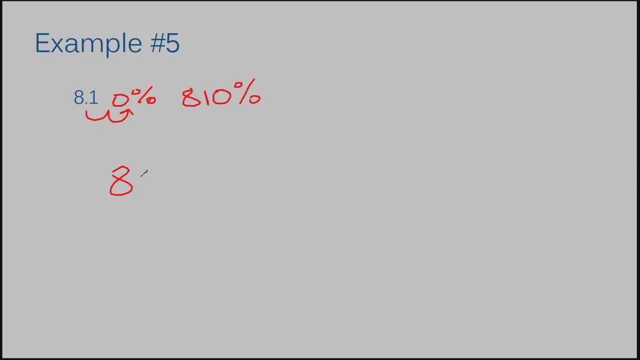 From the beginning. So it's going to be a mixed number. It's going to have a whole number of eight And then you're going to have your fraction portion. This is one tenth, So tenth is the position it's in. 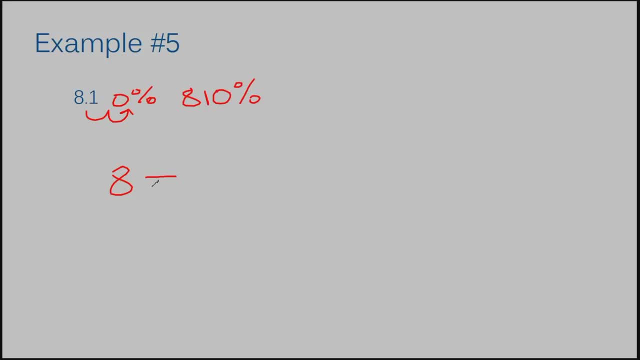 And that tells you what your denominator is going to be. It's going to be a tenth, Which means ten, One And ten. This cannot be simplified, So the three different forms of my number are Eight And one tenth. 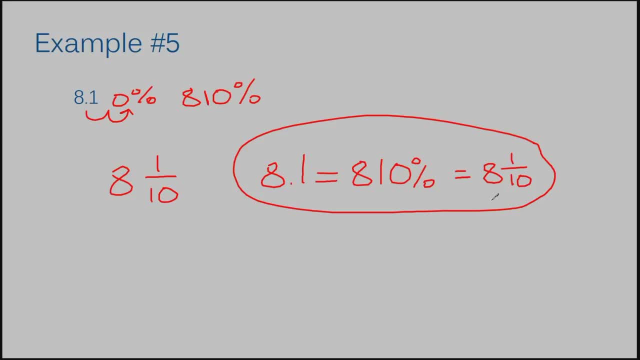 Eight hundred ten percent And eight And one tenth. Let's move on to example number six. Example number six: Ninety two percent. If going from a decimal to a percent Requires you to move the decimal two spaces to the right. 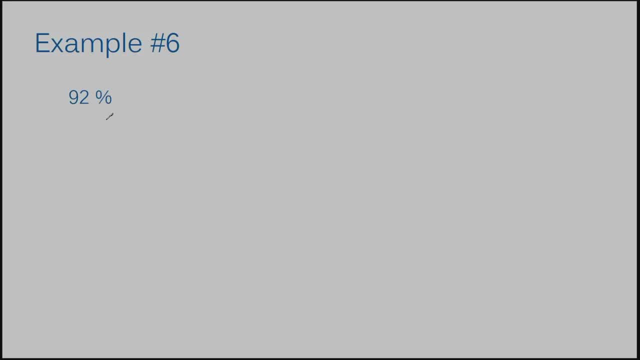 You may realize That the opposite is going to be true. To take a percent to a decimal, And it is. You take your decimal And you move it two spaces to the left. The decimal form of ninety two percent is: 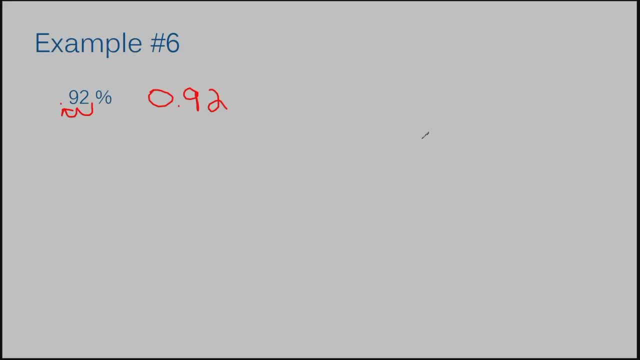 Ninety two hundredths To go from my decimal to a fraction. I need to remember how I properly say that decimal Ninety two hundredths ends with the word hundredths, So that gives you a hint right there. Hundredths mean make your denominator a one hundred. 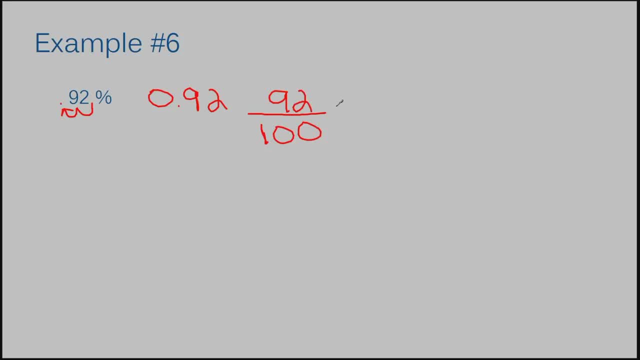 Ninety two will be your numerator, And this can simplify. I can divide the numerator and the denominator by four. When I do that, I get Twenty three over twenty five, Twenty three over twenty five. So my three numbers are: 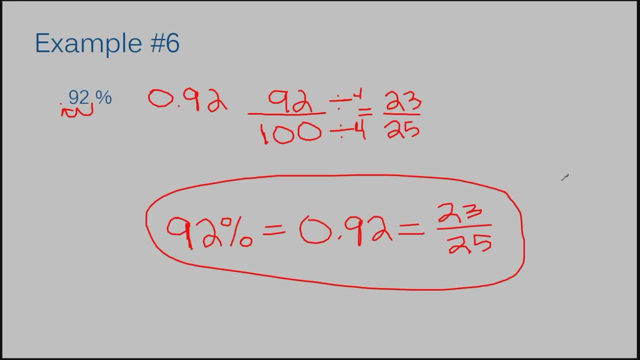 Ninety two percent, Ninety two hundredths And twenty three over twenty five. Let's move on to example number seven. I have one hundred fifteen percent. I take my decimal And move over two spaces to the left. This time it ends between two numbers. 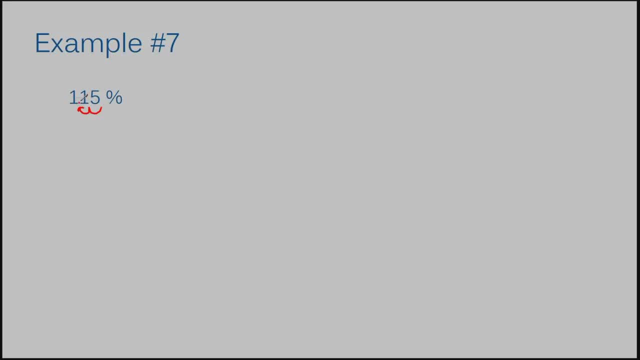 The two ones. So that means one And fifteen hundredths Is my decimal form of one hundred fifteen percent, To make this into a fraction. I remember I have a whole number, So my fraction is going to be a one and something. 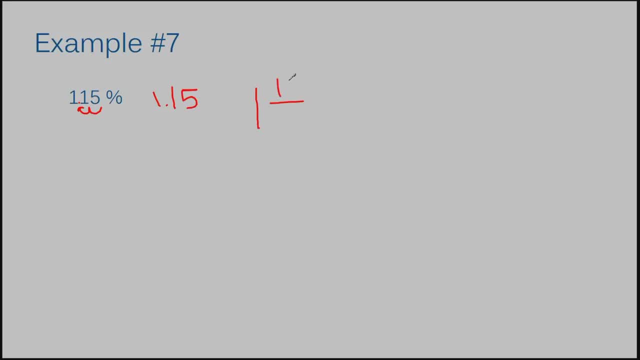 And we have fifteen hundredths. So that means fifteen Over one hundred. That can simplify. I'm only going to simplify the fraction portion. The whole number just remains the same. I'm dividing both the numerator and the denominator by five. 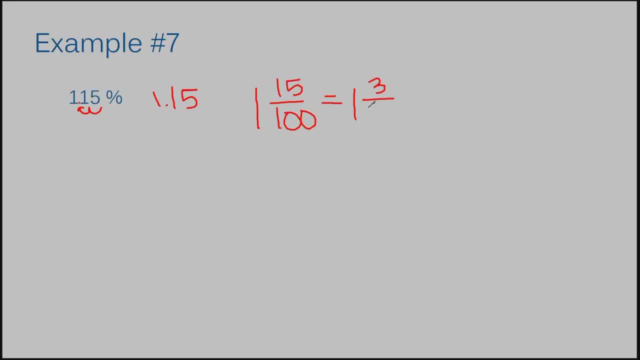 Fifteen divided by five is three, And one hundred divided by five is twenty. So one hundred fifteen percent, One and fifteen hundredths And one and three twentths Are all the same value And they are my answer. for example, number seven.